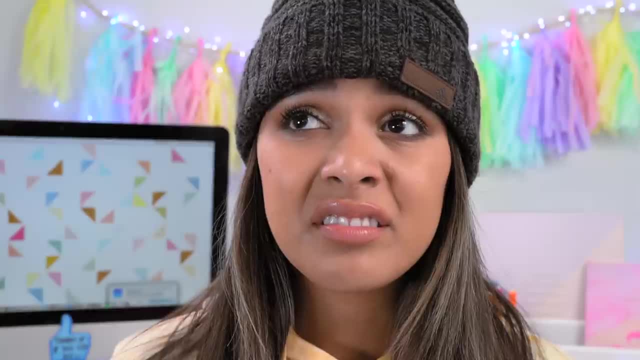 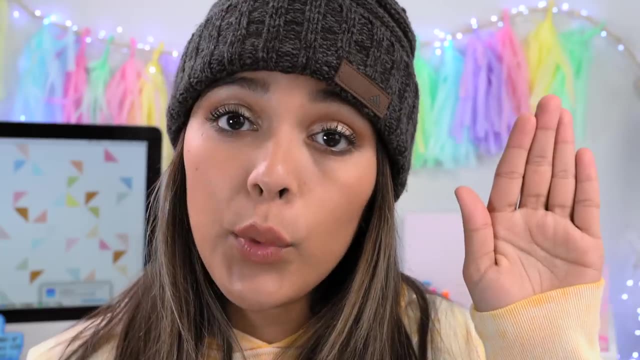 Hello there, I'm Natalie and I was an unorganized mess. I like to say it's the artist in me, but it's not. I'm a messy person by nature. Raise your hand if you're an organized. In this case. give this video a thumbs up. 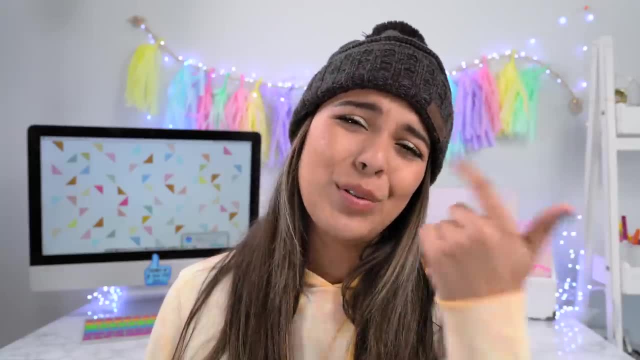 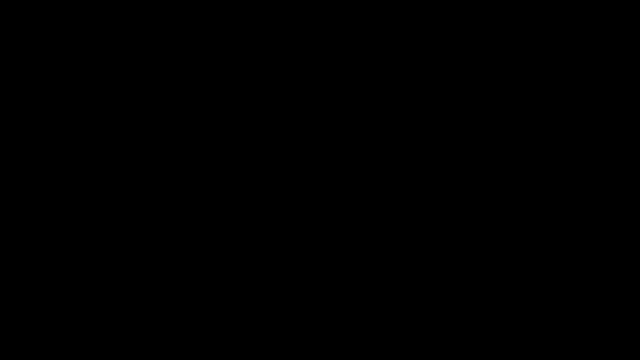 It's okay, I'm not gonna judge you, We're just gonna bond on a whole new level. I'm gonna show you the best DIY organizational hacks to keep your room, bathroom, kitchen and desk area clean, Hold up. I'm doing a huge giveaway where I'm giving one lucky subscriber a Canon camera. 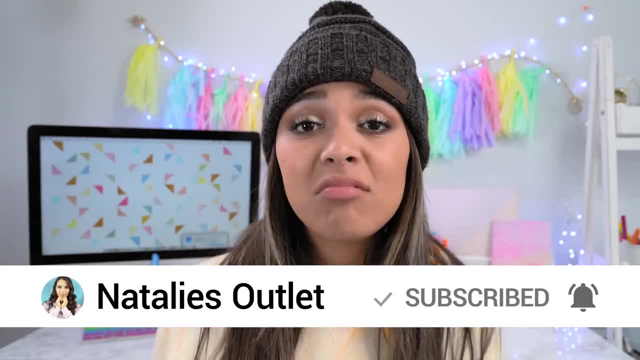 To enter, just subscribe and become a part of the family and that's it. It's that simple. I challenge you guys to get this video to 250,000 thumbs up. You guys have been beating every single challenge I've given you so far. 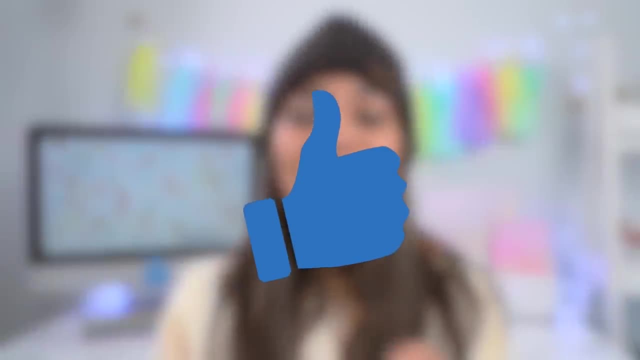 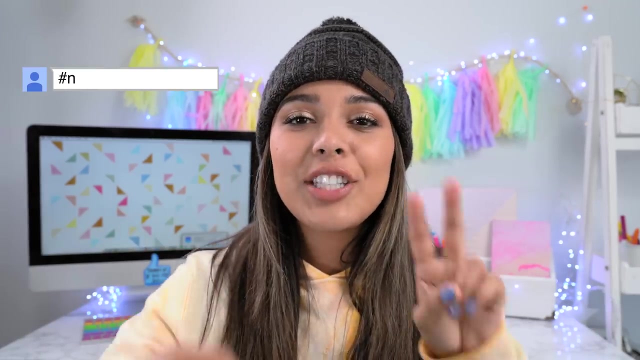 I dare you to turn this to this by clicking below and hitting that thumbs up. I want to give a huge shout out to Alili for watching my videos. Thank you so much. So if you want a shout out in my next video, just comment below hashtag: NatificationSquad. 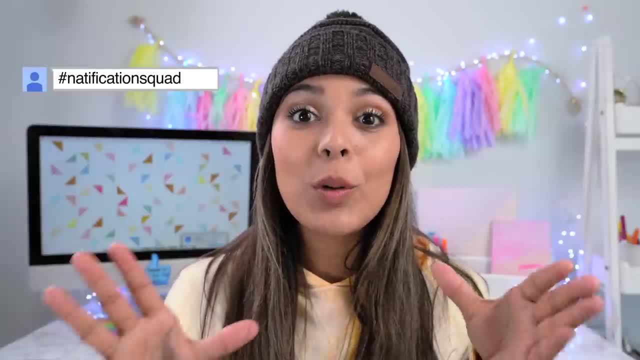 And if you're here within the first 30 minutes that every video goes live, I will be picking one of you, So make sure you're here early. Add me on Instagram, because I'm currently doing a huge giveaway where I'm giving away my favorites. 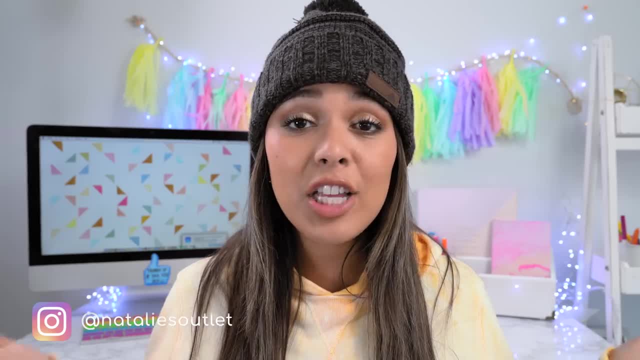 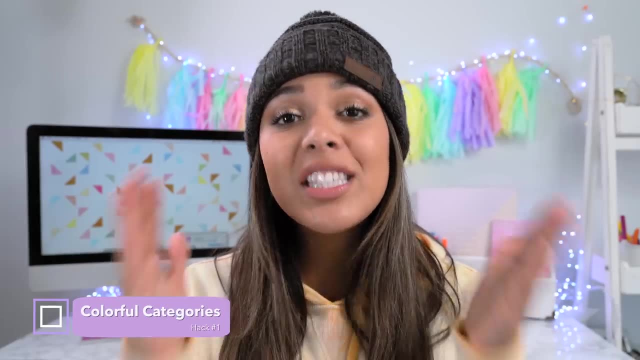 Polaroid makeup, stationery brushes- basically Natalie's essentials to you. Let's get on to the video. So this hack is to help you keep your desk clean. I want to say I'm not organized unless I have a system in place. 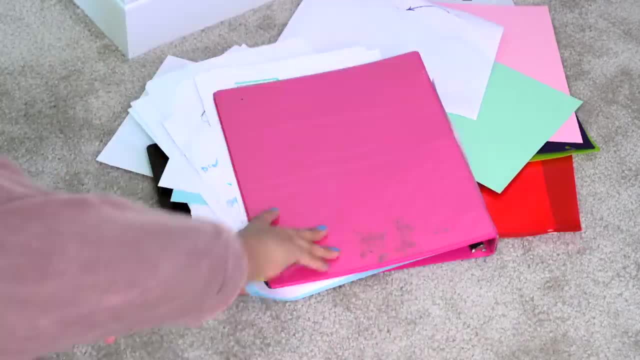 So if you're someone like me that just gets a bunch of papers and sticks them into a binder, whenever you need them, you open it up, you try to find what you need. you're not really helping yourself. You're wasting time. So let's get a system in order. 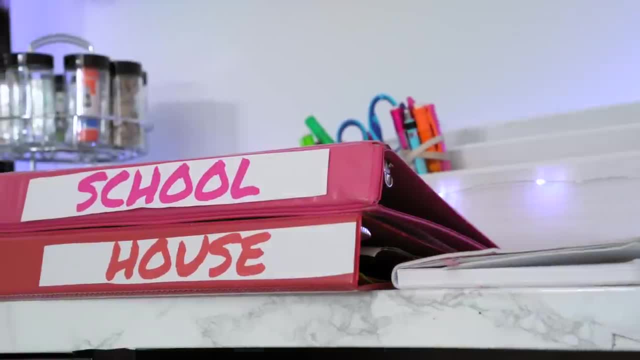 So my hack to you is to take a few colorful binders, categorize the binders So, for instance, you could do medical, you could do school, pets, homework, schoolwork, whatever you want, And that is a folder specifically for you. 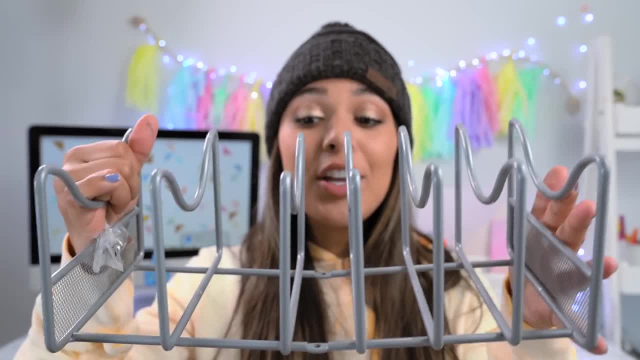 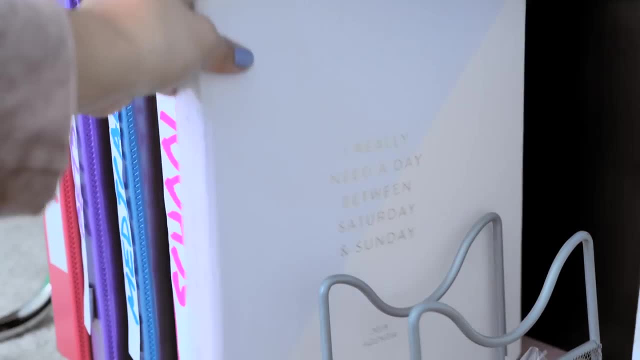 Specifically for that category. I'm telling you it's going to save you so much time. Also, if you get yourself something like this, which is actually used to organize pans in the kitchen, you can also use this as just an organizational tool for different binders for different books in your desk area. 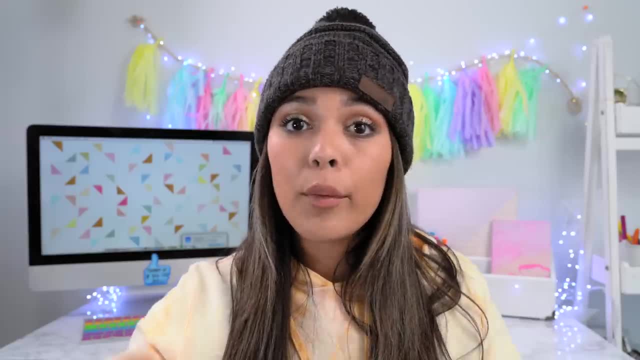 All you have to do is just print out a few different tabs, Just paste them on or glue them on or stick them inside the binder, And then there you go. You literally have a bunch of binders categorized. You can take one whenever you need in the specific category. 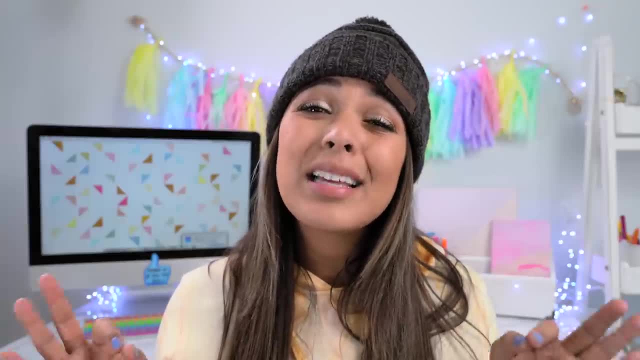 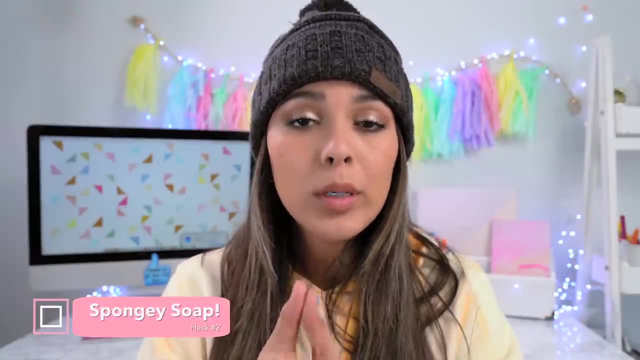 Open it up, Find what you need, Save yourself a lot of time And your room will be less messy And, trust me, your desk area will just stay clean. Since this is a cleaning video, you also got to clean yourself. This bathroom hack is going to save you so much cleaning and also so much soap. 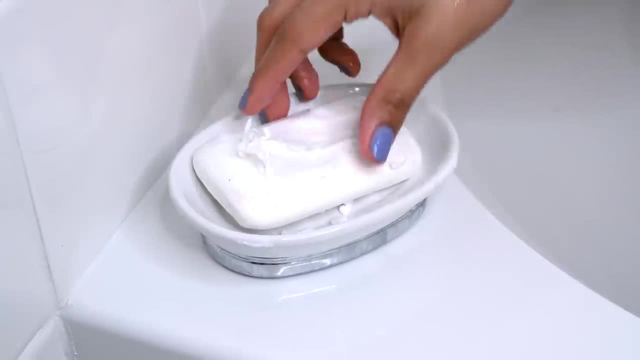 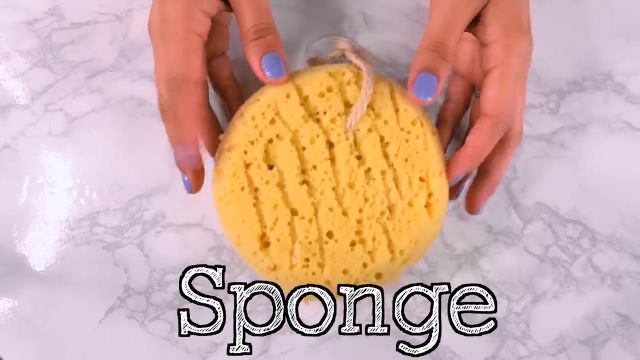 I know a little weird, But if you've ever experienced your soap drying onto the little soap bar that you place it on top, it looks nasty, it looks gunky, It just it doesn't look cute. So I recommend you guys to get a sponge similar to this one. 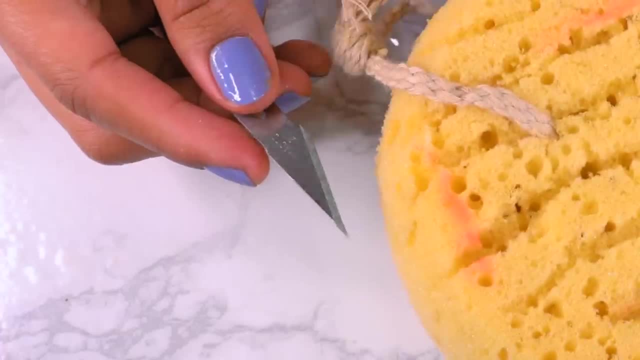 You're just going to put the soap over it, You're going to trace it, You're going to cut it And then you're going to create a nice little mold for the soap to go into. This is amazing, because you could use this as a sponge for all around your body. 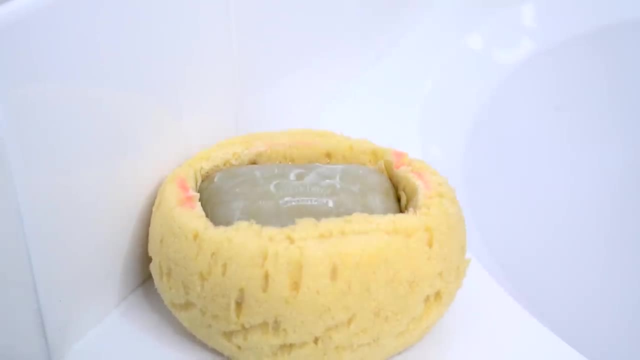 Or you can simply just leave it as a placeholder to put your soap every time you're done using it. You can actually do this. You can actually get the sponge and with it, just run it under water And you'll see all these bubbles just foaming. 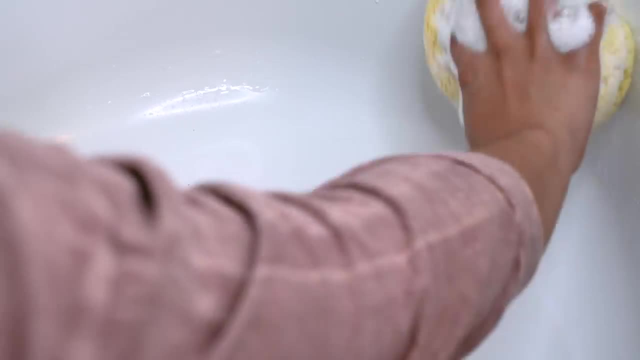 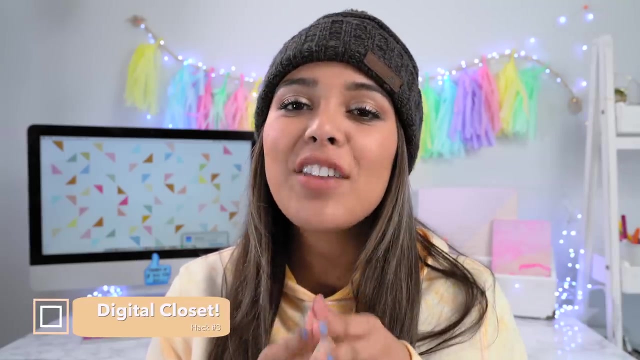 And you can use that to actually clean your bathroom. So there you go, Three hacks in one: You're cleaning, You are being cleaned And you are keeping your soap clean. It doesn't matter how much I've tried, I have never been organized with my clothes. 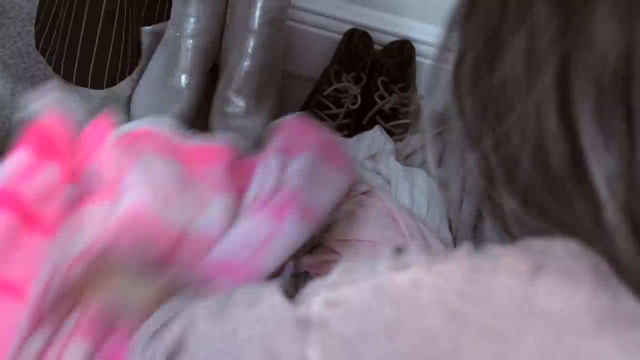 First of all, I can never pick an outfit. Secondly, I'm always running late And then by the time of it I'm just so overwhelmed and stressed that I'm trying to pick out certain pieces, And then I shove it back in there. 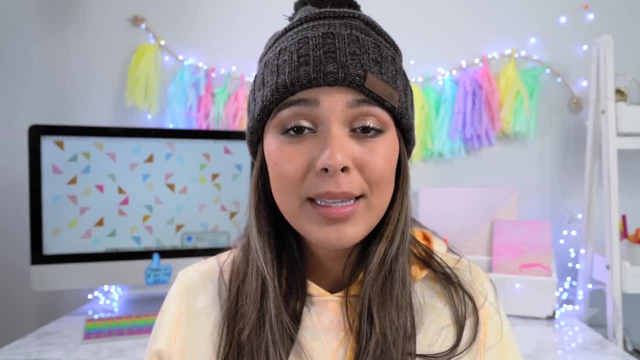 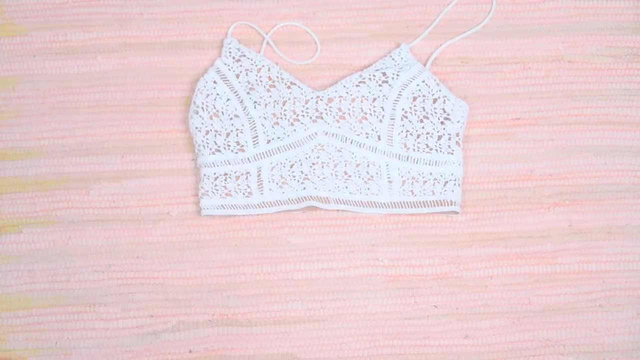 So what I would suggest is simply taking pictures of your favorite pieces, or even your new pieces. Just take an iPad or your smartphone And simply take a picture of your clothing On the floor. lay your clothes flat so that you can create a very aesthetically pleasing flat lay picture. 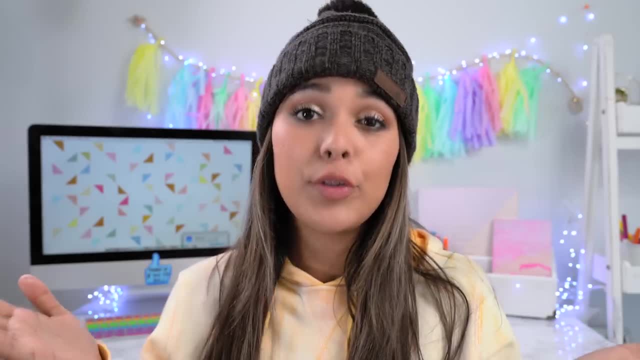 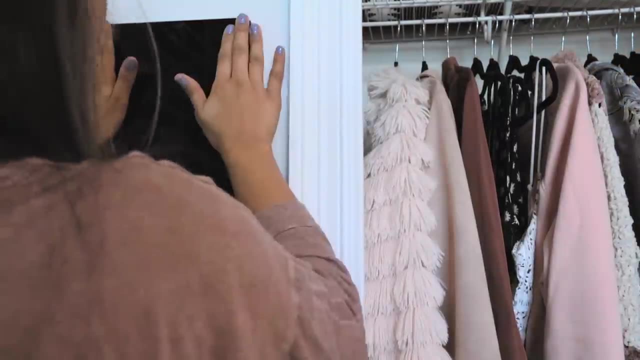 And then with those pictures, you can just create a notebook inside your iPad or whatever you're using And taking whatever device you're using, just take one of those little sticky tabs and stick it to the back of the device And then place it on a wall near your closet. 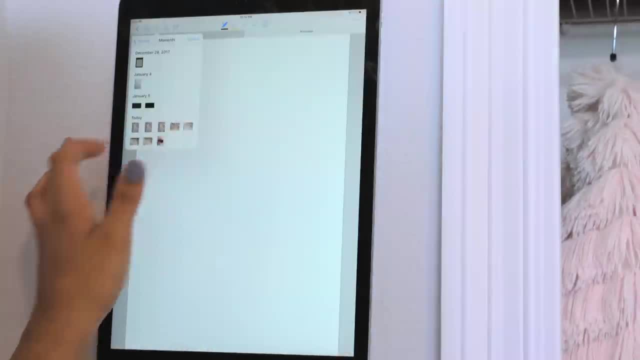 That way, right before you get dressed, you can always just look through it and decide on what you want to wear And simply start to bring pieces together and see what looks good together. Just mesh it, Get really creative. It's really inspiring to see the different pieces come together. 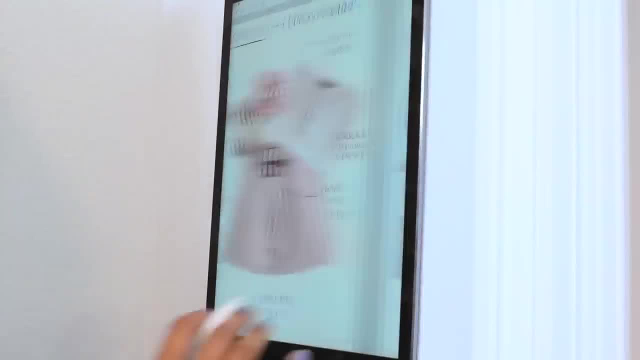 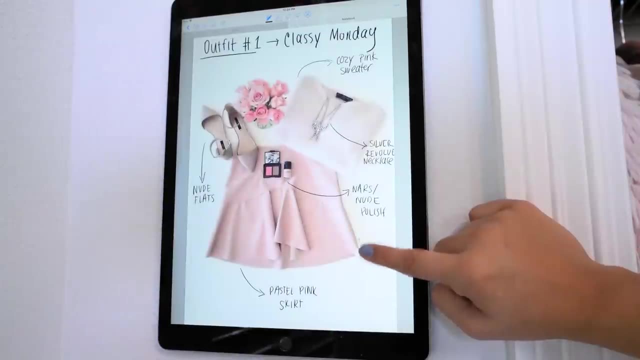 And importing pictures, You can see if that matches with the shirt and the accessories and all that jazz. And then you can actually save those outfits, Specify which day you want to wear them And what type of feel you want to feel, So, for instance, you can have like a casual day. 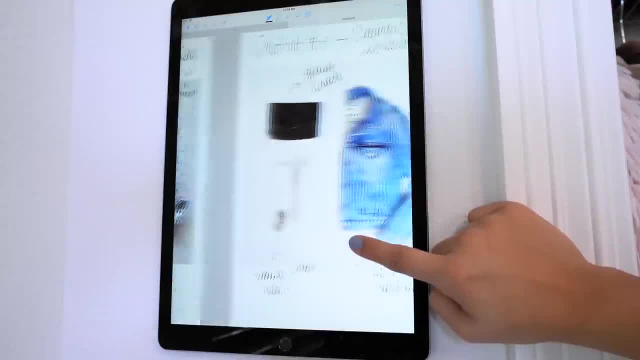 You can have a really classic, chic day, A sporty day. It's a great way to look at your closet from a different point of view And it's going to help you so much. It's helped me a ton. Every single time I do this, I'm much more satisfied with my outfits. 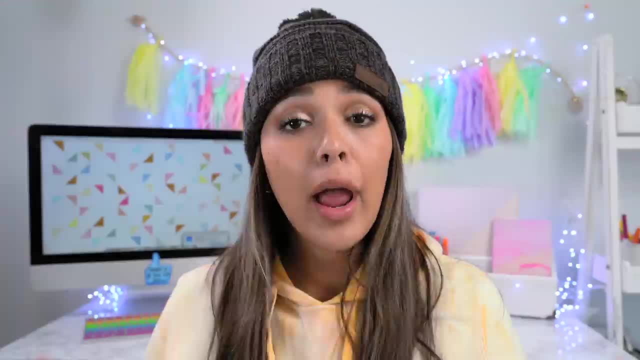 I feel more confident And I'm like dang girl, I'm working it. I'm a saucy girl, Meaning I like my sauces, But whenever I'm in my kitchen, in my refrigerator there's just so many different sauces. 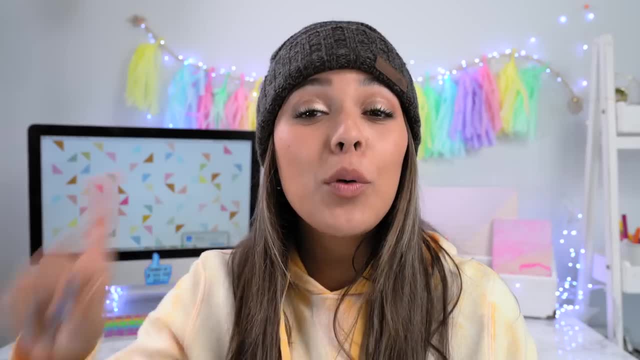 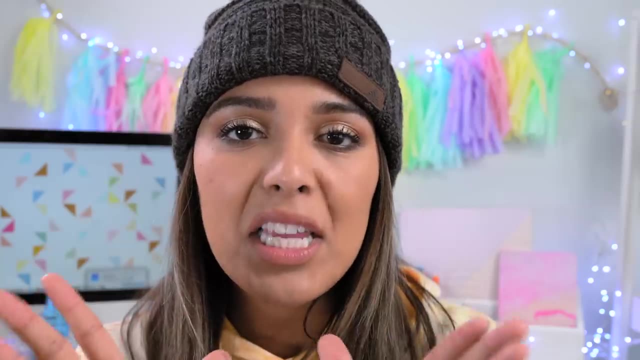 I'm not inspired to eat a salad man And I have to be healthy this year, But I will recommend this hack for you so that you're not searching through all your cabinets and refrigerator for all the different sauces And you can just keep them all in one sinked place. 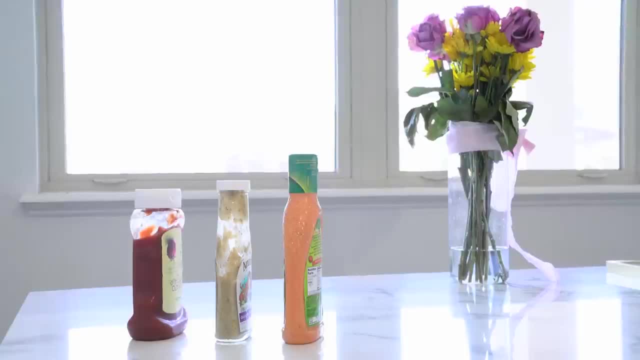 So simply get yourself an egg carton. That's all you're going to need. You're going to get the egg carton And then, with all your sauces, just place them upside down onto the egg carton. It'll keep it nice and secure. 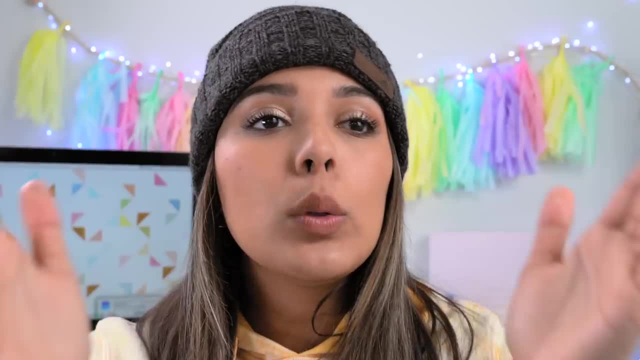 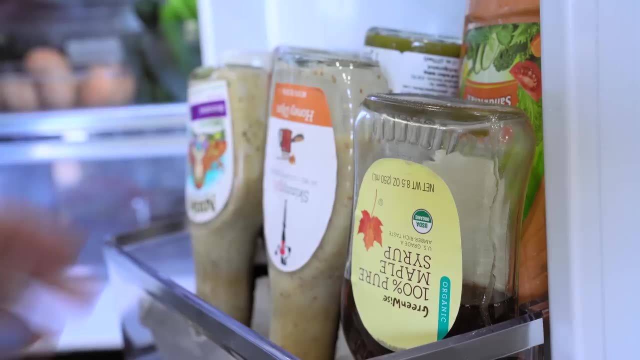 And then you can place that in your refrigerator And literally it's just beautiful. All your sauces will look beautiful, They'll inspire you to eat a salad or get saucy, And they won't move around. They'll literally be in one beautiful place. 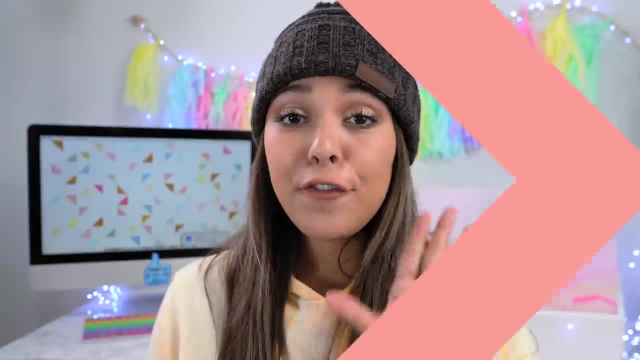 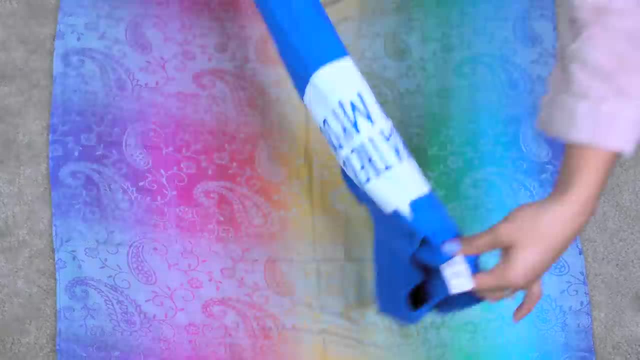 So much better. I've been eating my salads three times a week. For those of you, like myself, who continue to not know where anything is in your closet, trust me, I feel your pain. With shirts, specifically with t-shirts, you could do this. 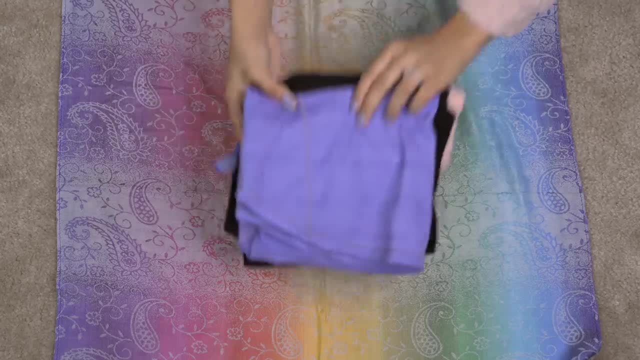 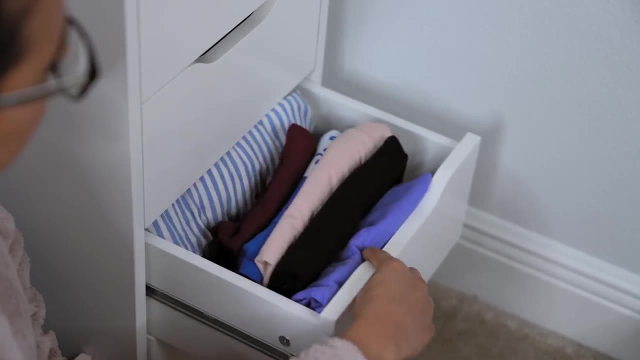 All you got to do is just fold a shirt like you normally would. But here's the trick: Instead of stacking your shirts on top like that, you're going to flip them over. What an interesting idea. So that way, when you open up your cabinets, you're not searching this way for all your shirts. 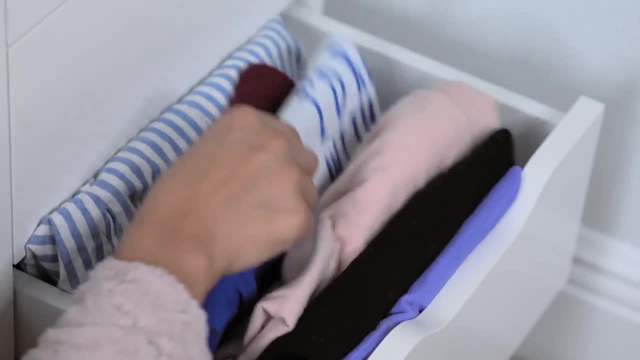 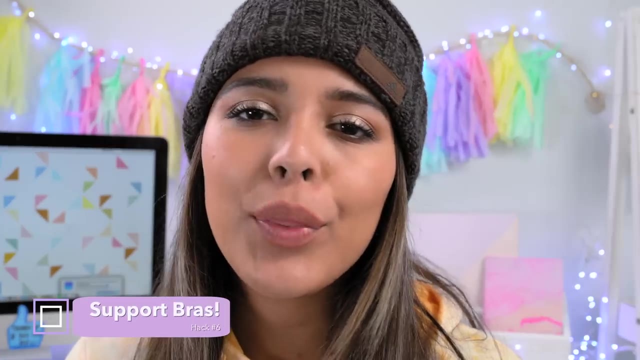 Instead, you're literally looking directly at all of them. It's literally like looking through file cabinets. I can just pick it out. It's so simple. Game changer, Ladies, your bra supports you, So we got to support the bras. 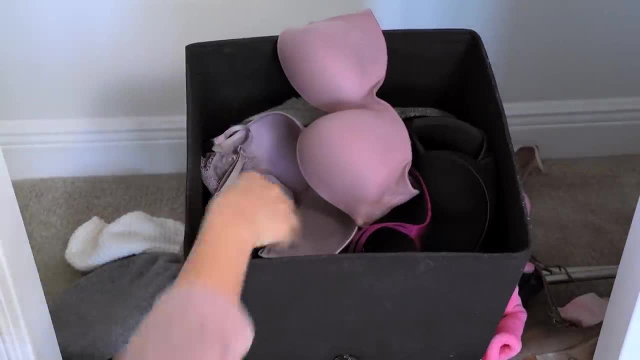 For this hack. instead of putting all of your bras into one cabinet, or however it is that you store them, we're going to hang the bras- Revolutionary, I know. So taking a hanger like this that has a lot of different slots. 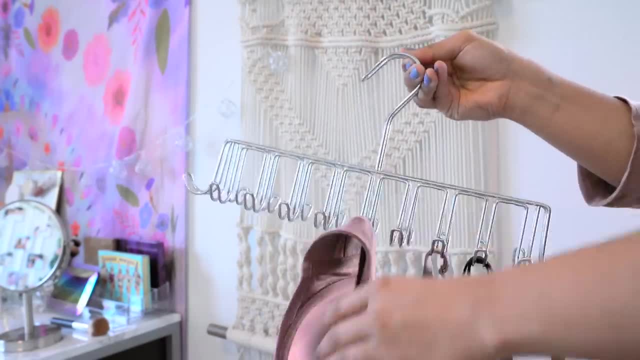 you can literally just grab a bra and hang it on there. It will not budge, It will not fall off. It will make it so much more easier for you if you have to get dressed and you need a specific type of bra. So let's say you're looking for strapless bra. 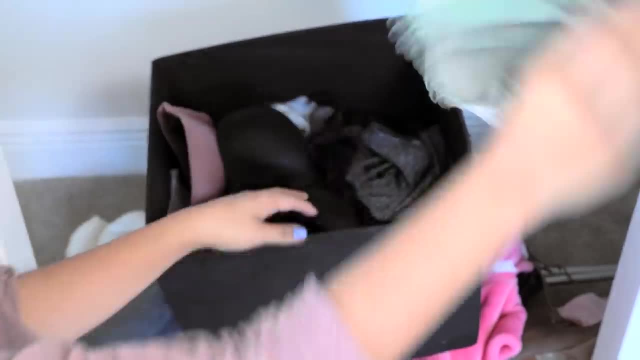 You literally see it So much easier than seeing your bras distorted, And then you're trying to grab them And then you're like: I don't like this bra, I hate this bra, I hate this bra. And for guys, you can literally do the same thing with your boxers. 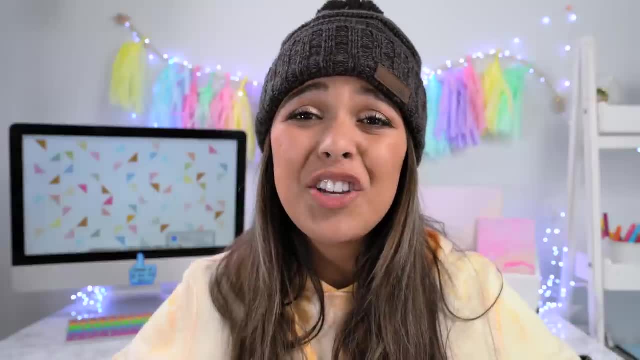 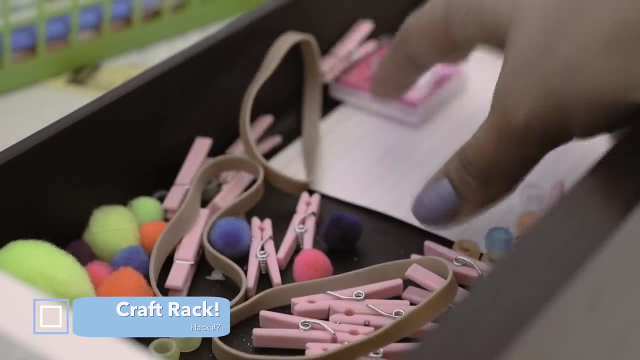 It's going to help you stay so much more organized, Your closet is going to be so much more clean And you're going to not waste your time looking for a specific type of bra. This hack is literally one of my favorites If you experience tragedies like this one. 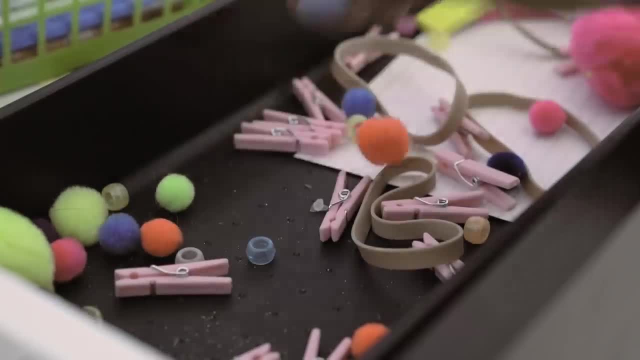 where you literally throw all your DIY craft supplies into one cabinet, or just your desk office supplies. fear or not, I have a solution for you. All you're going to do is get a spice rack- Yep, a spice rack. It looks pretty cute. 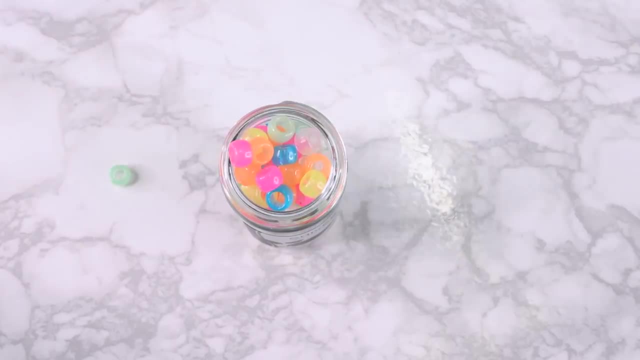 You're going to dump out all the spice. You're going to add anything, Anything you want into it. You can add rubber bands, You can add pins, staples, note cards, glue, thumb tacks, pennies, construction paper. 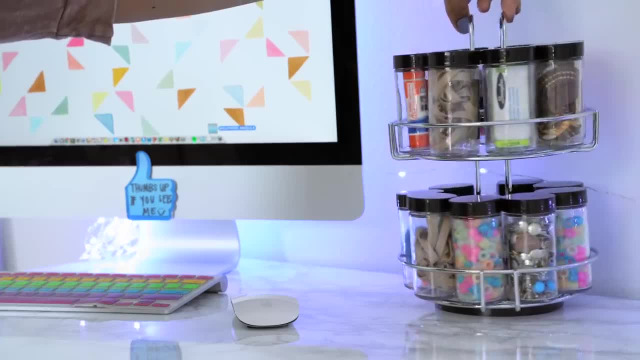 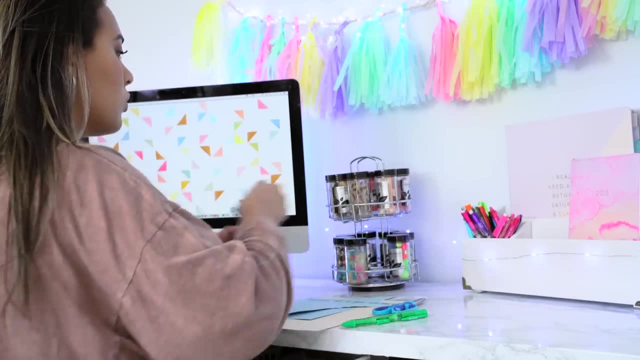 tape literally anything that you want, And it's so nice to have this on your desk because it doesn't take up too much room. You just got to twirl it and spin it to see what you need. It makes it so much more fun to create and get crafty and just have all your supplies all in one place. 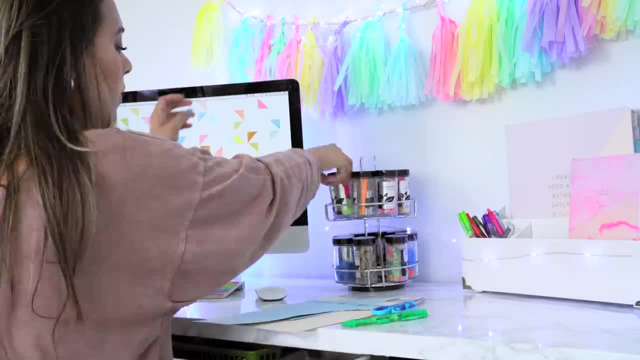 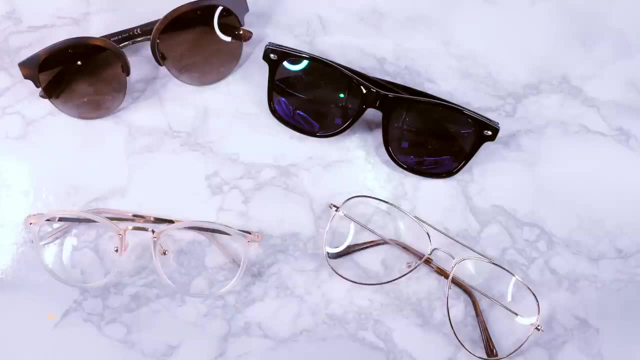 Highly recommend you guys to try out this one: Super simple, inexpensive and super effective. All right, So you're into glasses, but your glasses are always everywhere. Now, glasses can be a very delicate thing where, if you don't store them right, they can go bad. I recommend you guys to just get a hanger. Put that hanger anywhere that you want. You can even hang this on your wall really nicely, or you can just leave it in your closet And just hang your sunglasses. 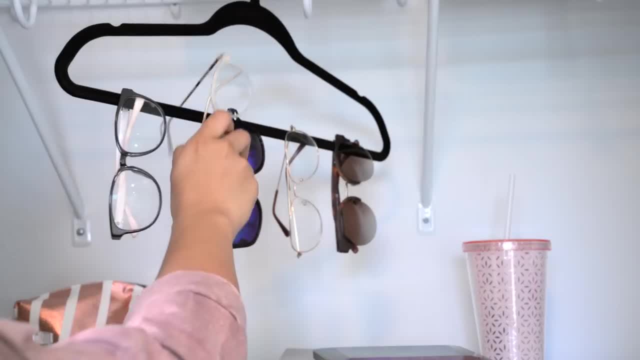 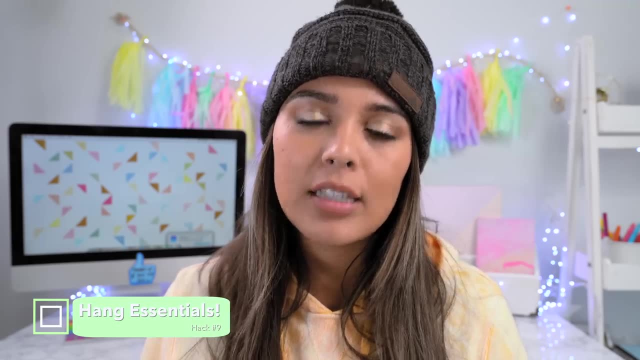 Hang your glasses. This is going to help you not only keep your glasses organized, but just know what you have and then wear it out. Get stylish, Get crafty. This hack is specifically for bathrooms- to help you keep it organized If you have a lot of products that you absolutely love but you're just kind of looking through. 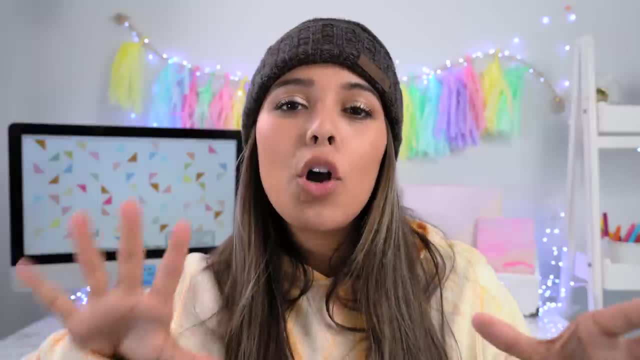 shelves. you just don't know where anything is. why not put all of your daily products in one little place? So we're just going to DIY a really nifty little place to put all your stuff. We're going to call it all of your daily essentials. 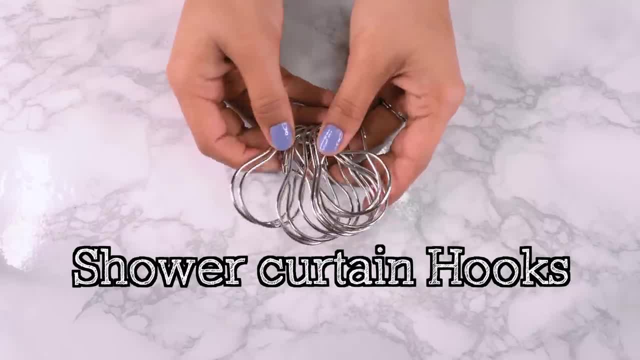 Using some pins and shower curtain, we're going to create a really nifty DIY. So you're going to take a shower curtain holder and then, with the pins, just tie it around and lock it into place And then pin your favorite products onto that. 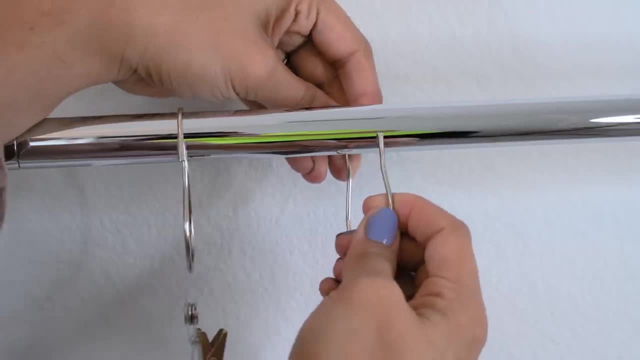 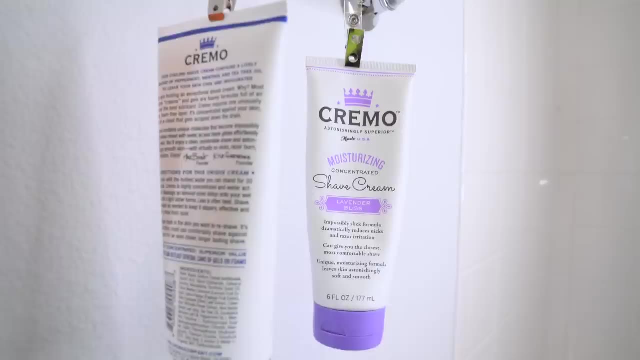 Then you can simply hang your favorite products and they're all going to be aligned in one place that you can actually see, that you can use on a daily, as opposed to just going through all these cabinets and looking for all the things that you already use every. 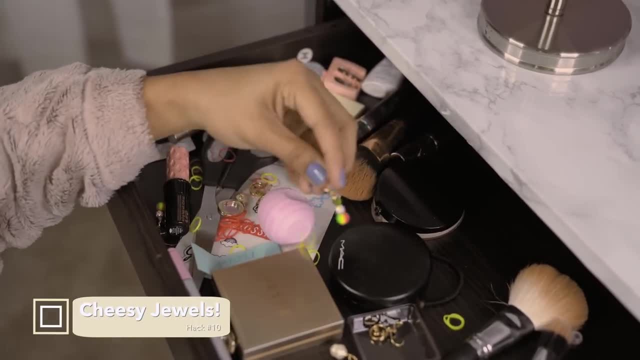 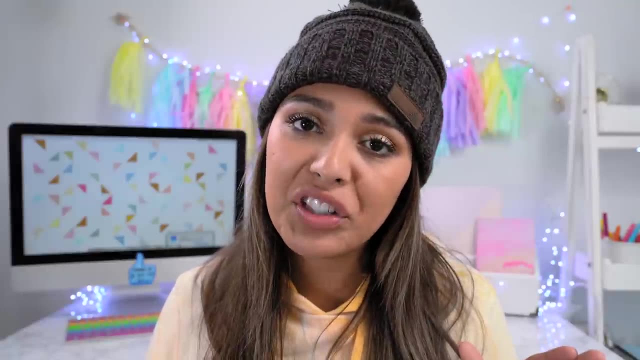 single day: Earrings, Earrings. I have lost so many earrings and I don't even use so many earrings. You literally see me using these earrings every single video. But if I had known about this hack, I would not be wearing these earrings every single. 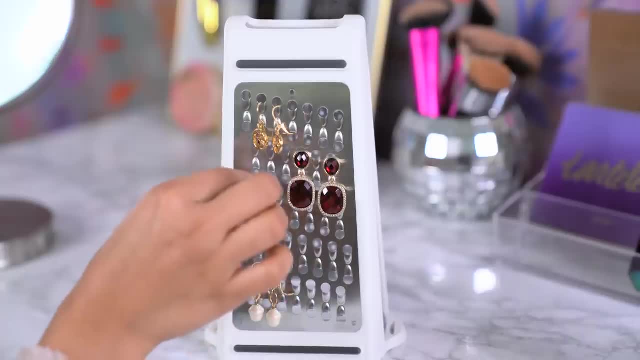 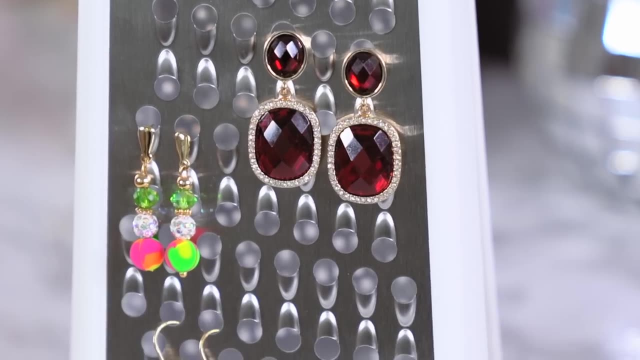 day. So all you're going to do is take a cheese grater. You're going to use this as a placeholder for your jewelry. It is so simple, It is such a life changer. Literally, just take all of your earrings and place them into one place. 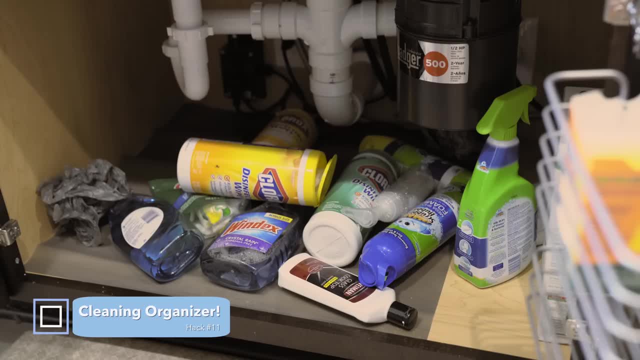 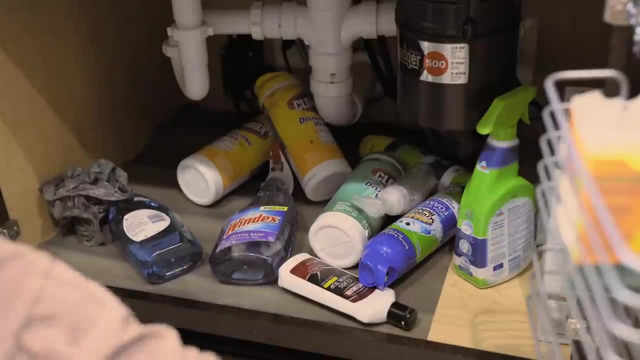 And there you go- Earrings for life. If you have a bunch of cleaning supplies or detergents just dusting away in cabinets- isn't that ironic? Then this hack will help you out. Instead of putting your cleaning supplies in a place where it is uninspiring- it doesn't? 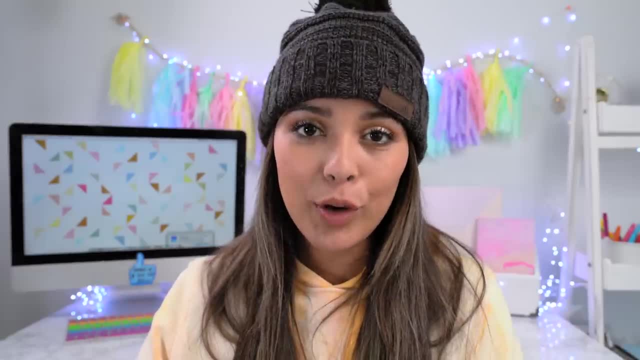 make you want to clean at all. Instead, just buy yourself a plastic shoe organizer. You should just store all your cleaning supplies. It's much more visually appealing. It's going to motivate you to want to clean. You're going to know where all your products are. 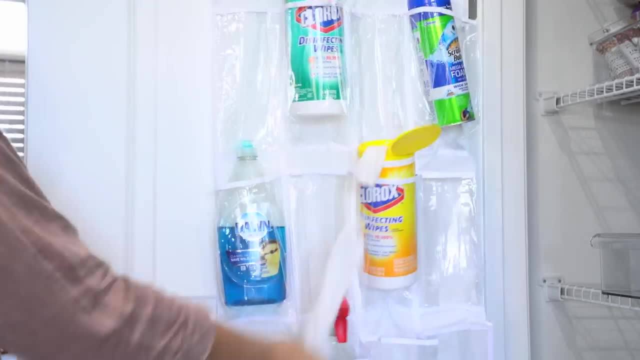 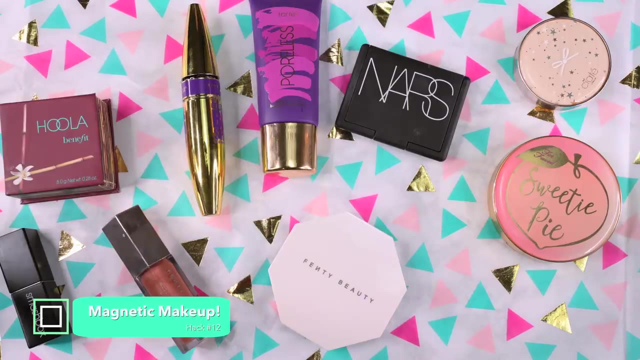 And then if you position this in a pantry or in a place like the laundry, where you can actually see it, it will subconsciously motivate you to want to clean. If you're a makeup junkie and all of your makeup is just messy and not organized, you. 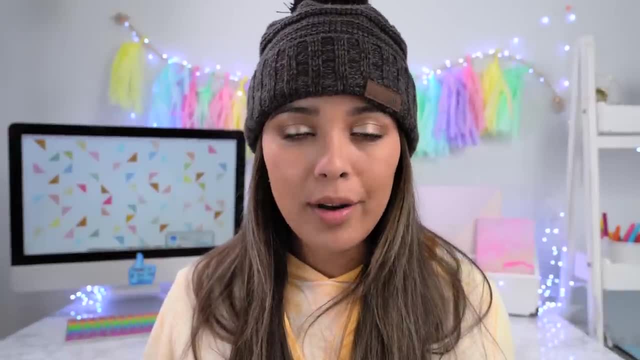 know you can have a lot of makeup, but you don't really use every single product every single day. So to simplify your life and make it much more organized, all you're going to do is take a really nice magnetic board and you're going to take your daily products that you 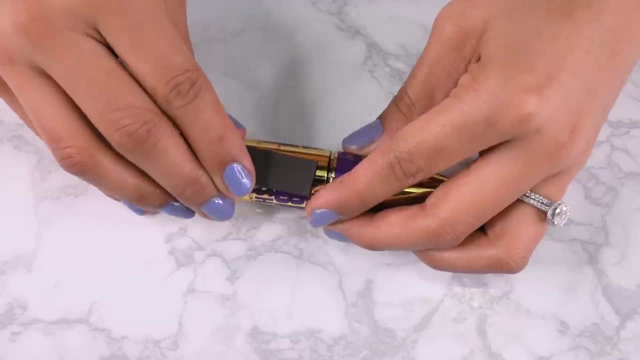 use every single day And then, using a magnetic tape, you're going to take your daily makeup products that you use every single day And then, using a magnetic tape, you're just going to snip it and cut a few And then just tape it to the back of every single product. 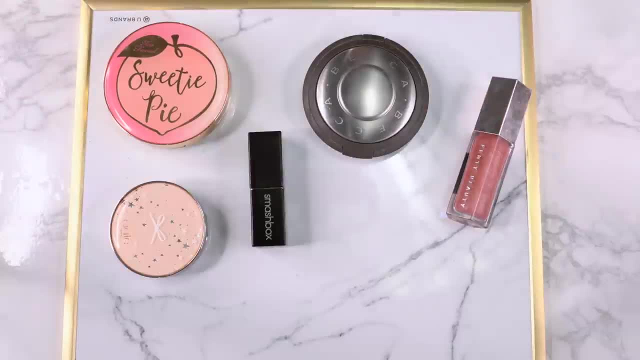 Now, when you're doing your makeup routine, you can literally move this board anywhere that you need: The bathroom, You could take it to school. if you need it, You could take it to your locker. You can move it away from your vanity. 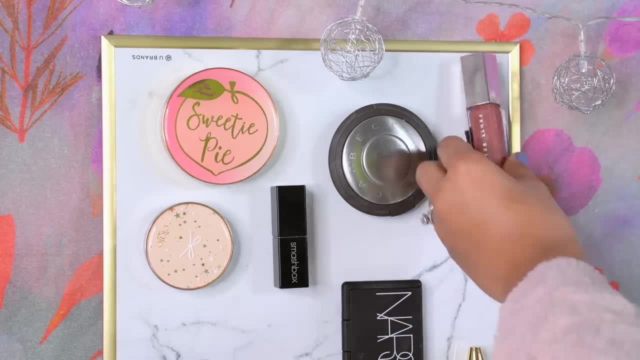 It's going to make it so much easier for you to just keep everything in one place- Really nice and organized, And you can switch them out. If those are no longer your daily to-go makeup products, then you can just switch them for other ones. 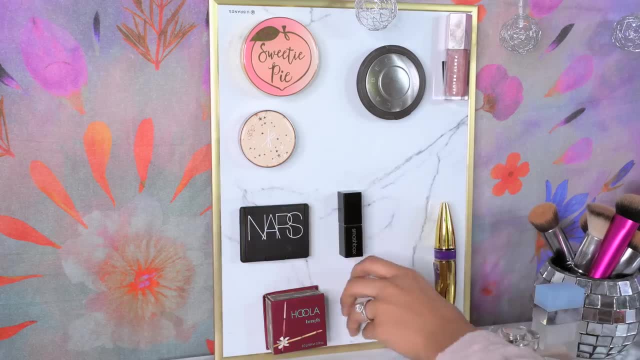 Just put some magnetic tape on them and there you go. Personally, it's made my makeup regimen so much simpler because I know which products I'm using on it daily. I'm not going through my makeup drawers like looking for the same thing that I use. 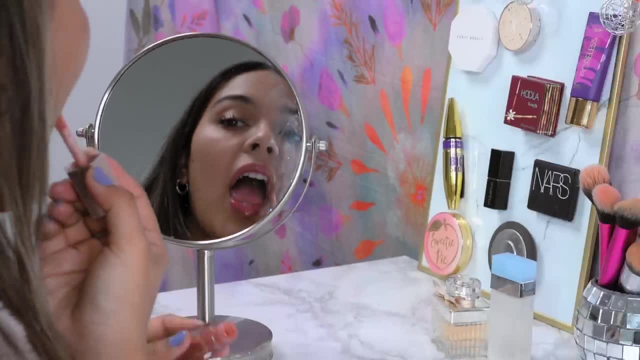 every single day, And it's a really inexpensive DIY. My room before Ugh And my room after- What a difference. If you enjoyed this DIY organizational hacks, make sure you give this video a huge thumbs up. Also, check out my last video right over here by clicking it, where I show you the best. 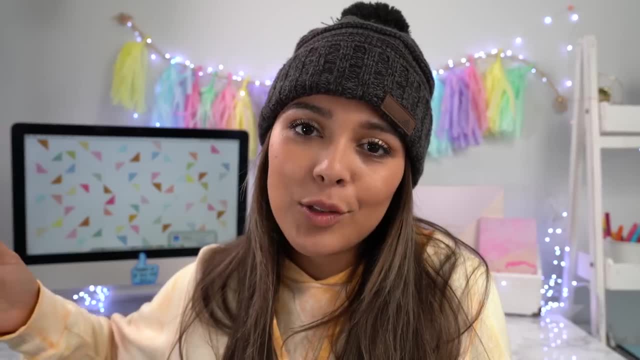 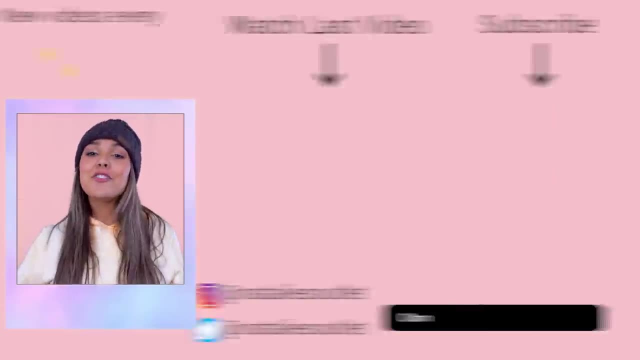 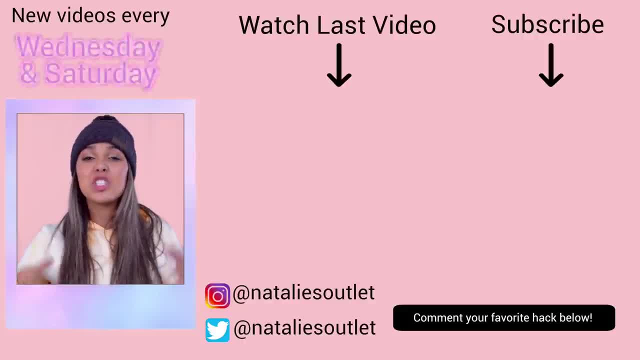 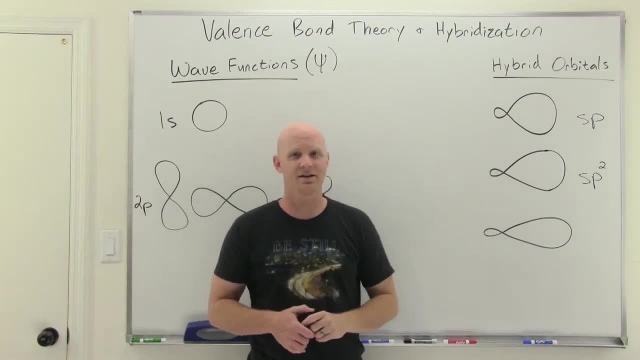 Valence: bond theory and hybridization. that is the topic of interest in this next lesson in my new organic chemistry playlist. So in this first chapter just a review of general chemistry and it's just a reminder of where we've come from and where we're headed. We just did lessons. 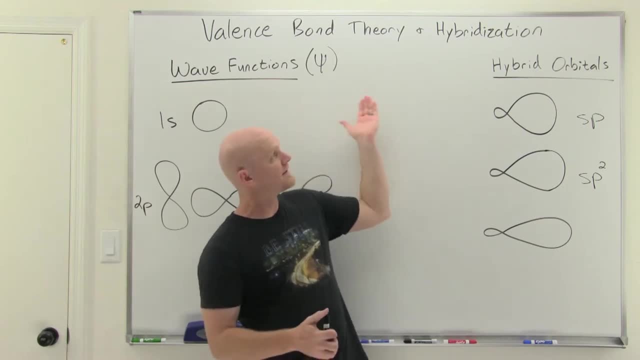 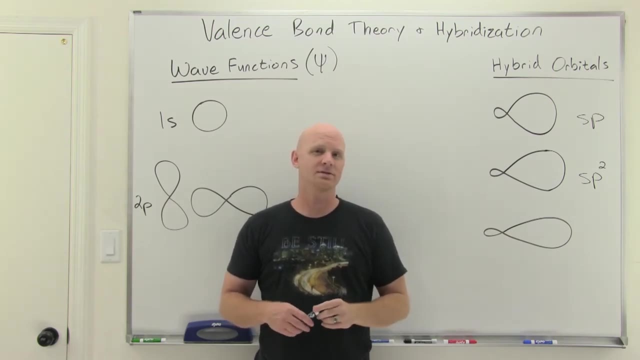 on Lewis structures and formal charges. We'll now hit valence, bond theory and hybridization, which will feed nicely into the next lesson on molecular orbital theory, And then, finally, we'll finish this chapter off with a lesson on polarity and a lesson on intermolecular forces. 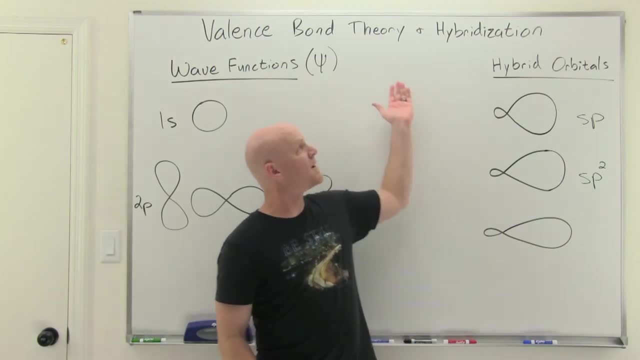 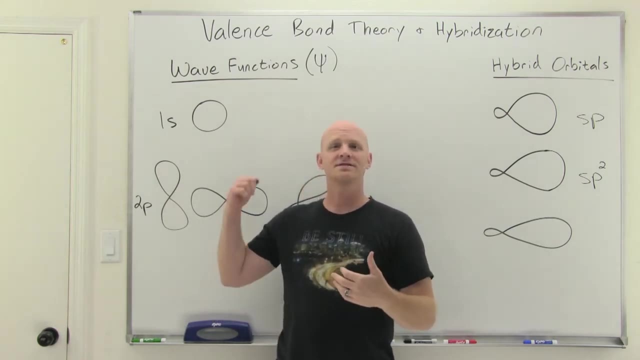 All right. so valence bond theory, So at the heart of valence bond theory, just talks about what creates a covalent bond. So we like to talk about the sharing of electrons and stuff, So. but this takes a step further and says that atomic orbitals are actually going to overlap. 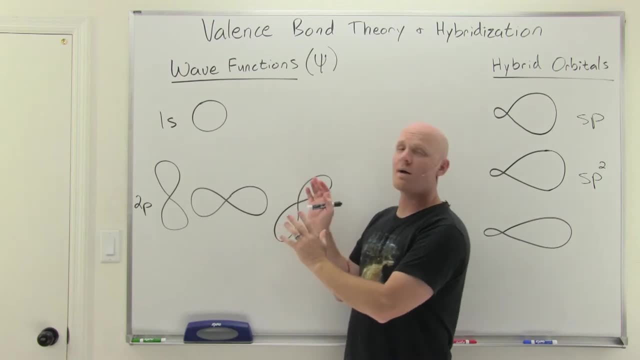 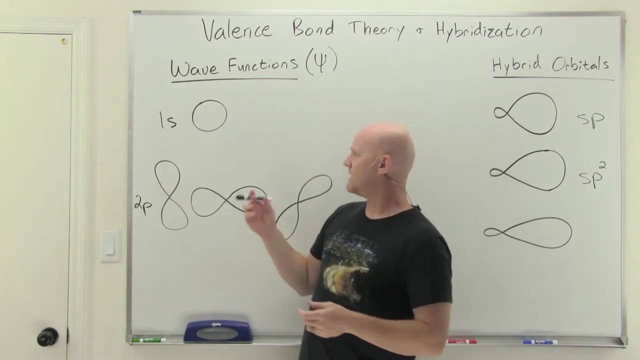 And that's where the electrons are going to be shared. So that's kind of the heart of it. So we got to remind ourselves what these atomic orbitals look like And want to look at first of all your 1s orbital, and it's just a nice spherical orbital, So a nice solid sphere like a bowling. 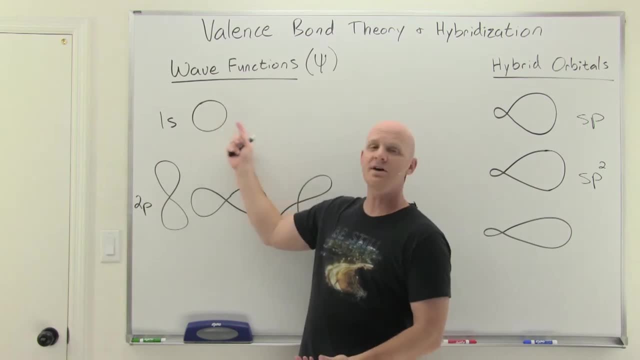 ball, not a basketball. So it's solid, So and it just gives you an idea of where you can find an electron: around the nucleus. So the nucleus at the center of that sphere, So, and somewhere in that sphere, at least to the 95% probability is what we're usually mapping. That's what the actual. 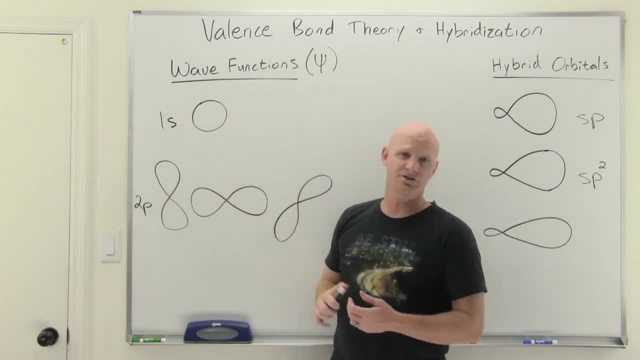 three dimensional equation would look like: And again we call those wave functions Now for a 2p, orbital. So these we say are dumbbell shaped And there is a what we call a node at the nucleus, And a node is just a place where the function goes to zero. Now you probably remember your sine.